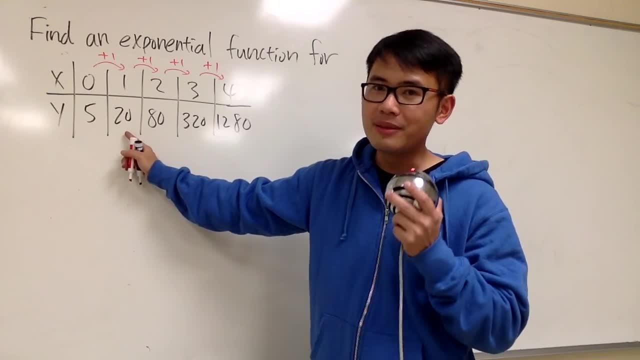 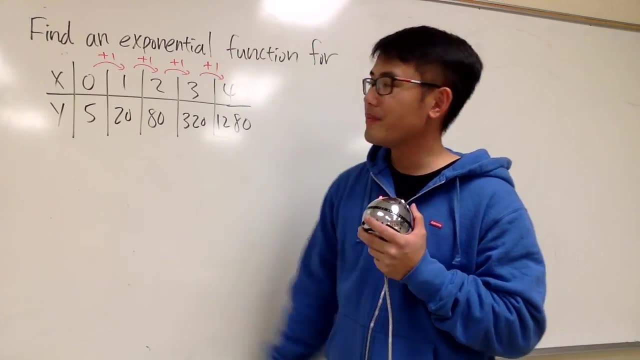 that's okay. from here to here. However, it doesn't work anymore from here to here. If you add 15 to 20, you get 35,. you don't get 80, right? So you have to look at this from a different way. Well, from 5 to 20,. 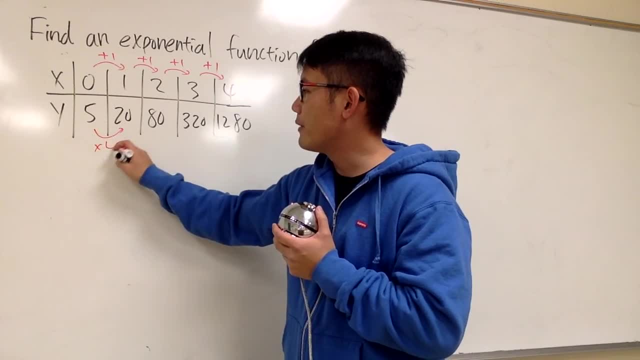 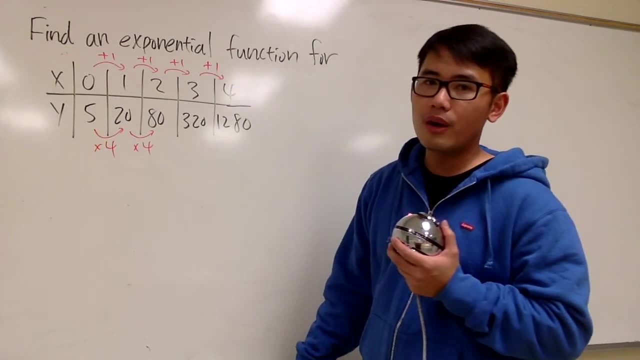 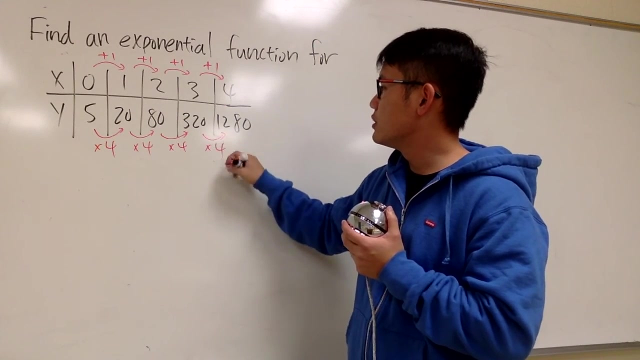 we know we can say: from here to here we can multiply by 4.. And then from 20 to 80, once again we can look at this by multiplying by 4.. And in fact that's the pattern: Each, every time we multiply by 4.. Check this out. 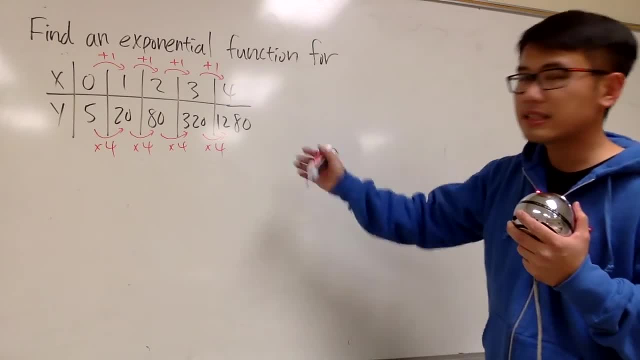 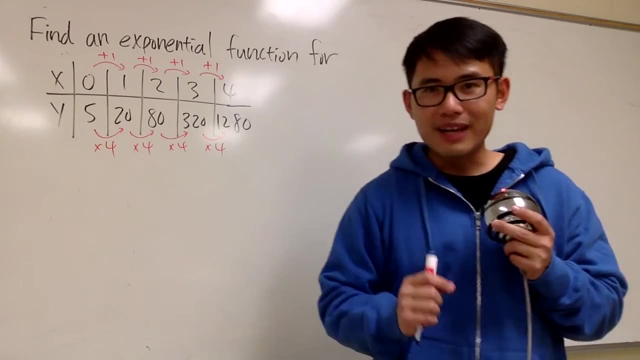 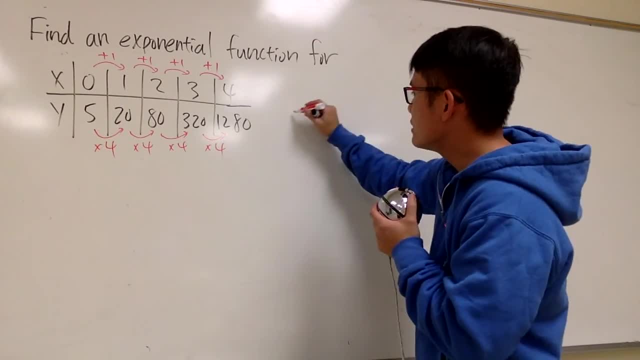 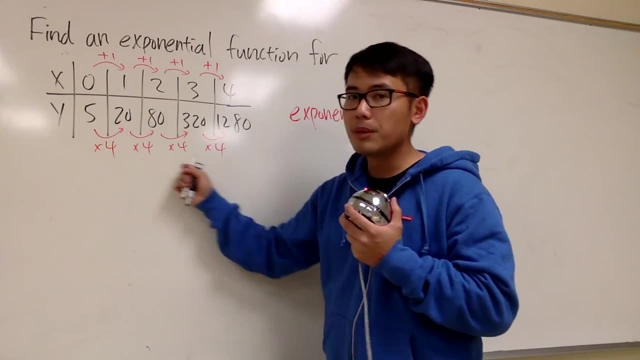 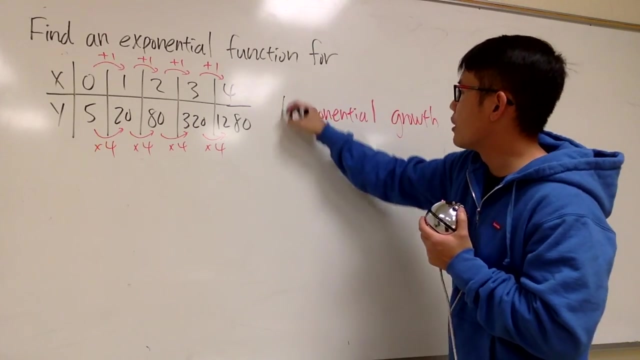 the same number over and over. In this case it is an exponential and, as you can see, the numbers are getting bigger because we are multiplying a number bigger than one Exponential grows because the numbers are getting bigger and bigger, and this is the difference between this table and the table. 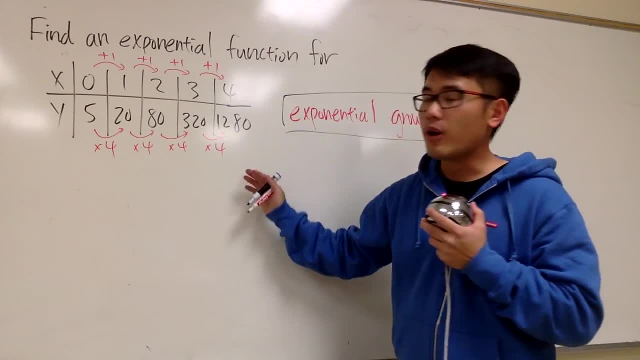 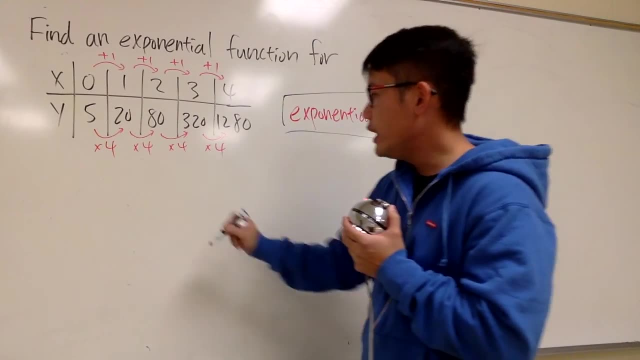 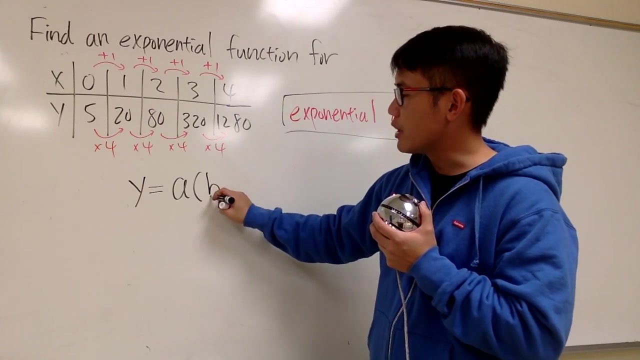 from question number seven. This is not easy at all because we're trying to find an exponential function for it. Let's write down the general form We have: y is equal to sum number a times the base for the exponential. Let me just put on b and put that in the parentheses and raise. 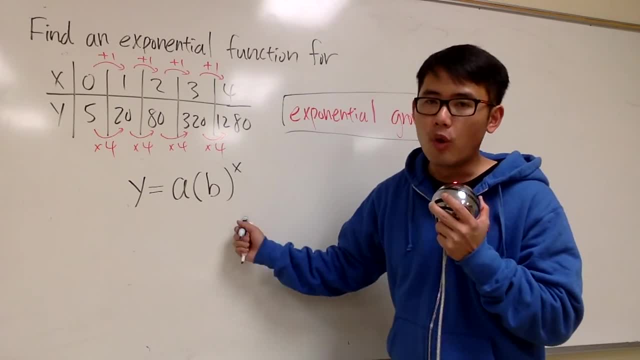 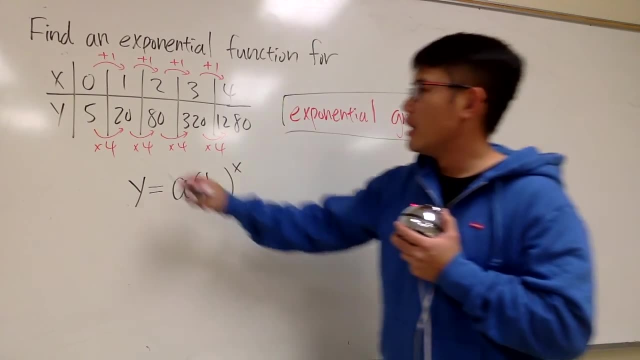 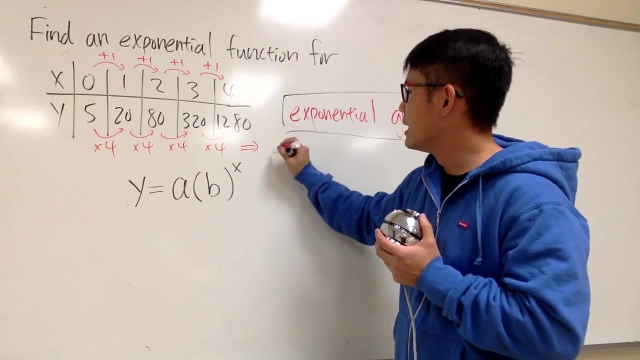 that to the x power. This is the general form for an exponential function and in fact we know one value already. This is four. We multiply the four over and over Right Here, it tells us that b is equal to four. We know this right away. That's the base. 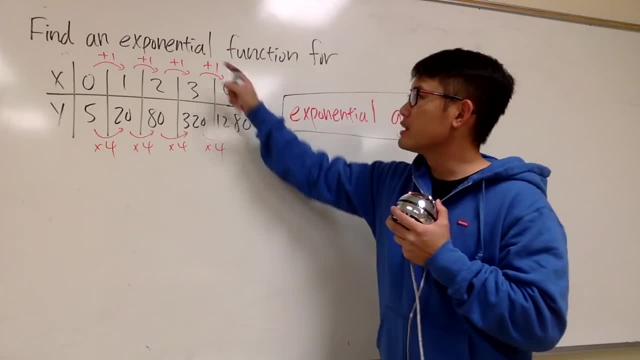 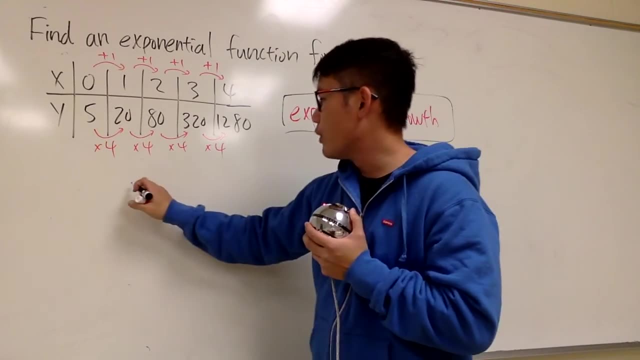 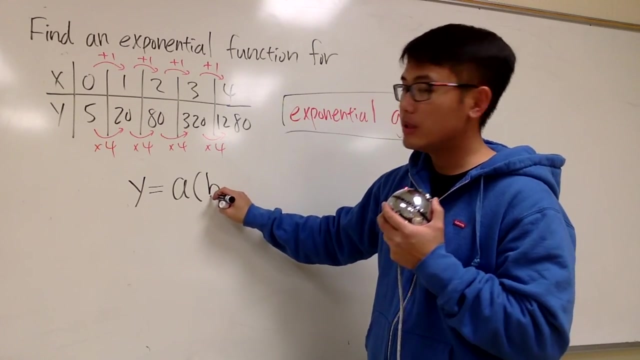 question number 7.. This is not 80 at all because we're trying to find an exponential pattern function for it. Let's write down the general form We have: y is equal to some number a times the base for the exponential. Let me just put on b and put that in the parenthesis. 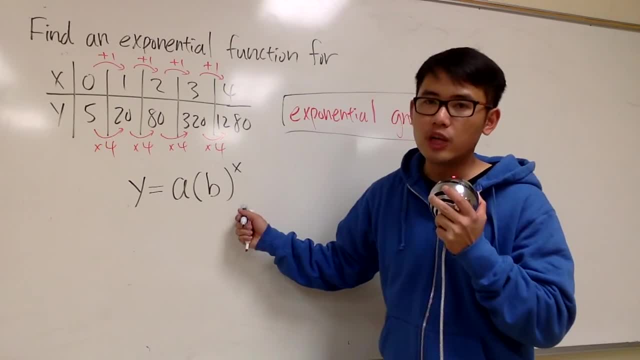 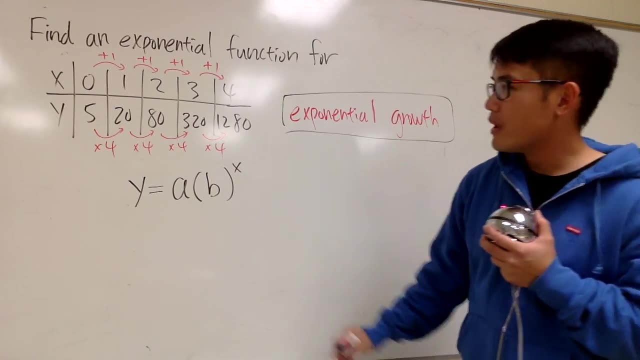 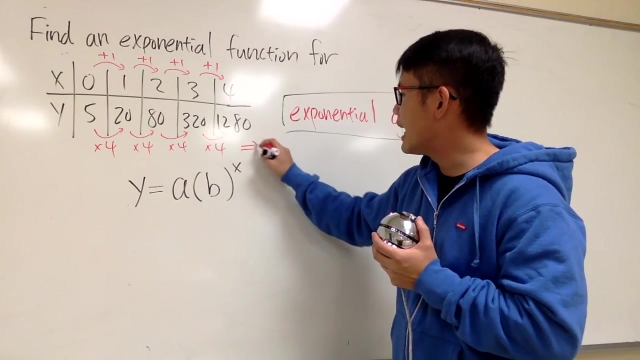 and raise that to the x power. This is the general form for an exponential function And in fact we know one value already. This is 4.. We multiply the 4 over and over right here, It tells us that b is equal to 4.. We know this right away. That's the base, okay. 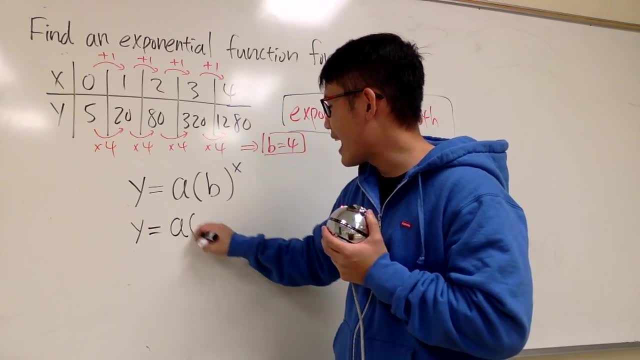 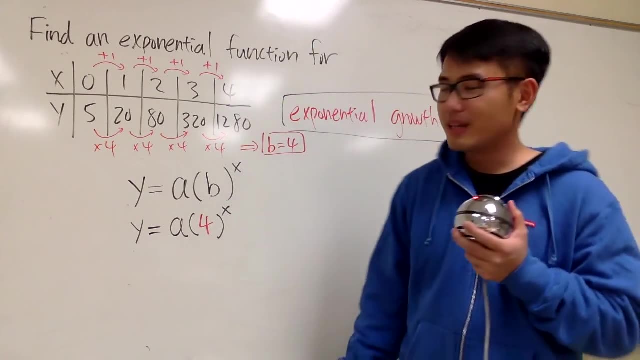 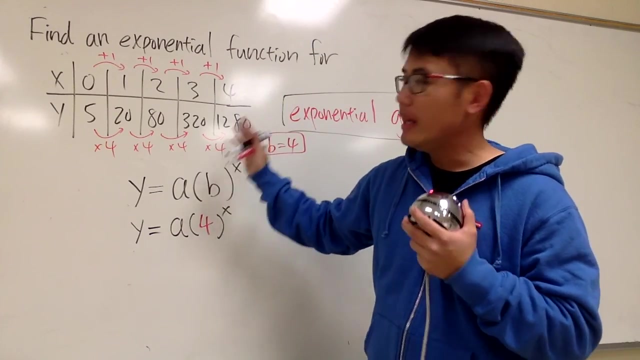 Therefore, you know, y is equal to a times b is 4, and then raised to the x power, like that. Well, one more thing will be done. What is the a value? Well, we have the x and y values right here. Pick a pair, Any one. I can use 2 comma 80.. 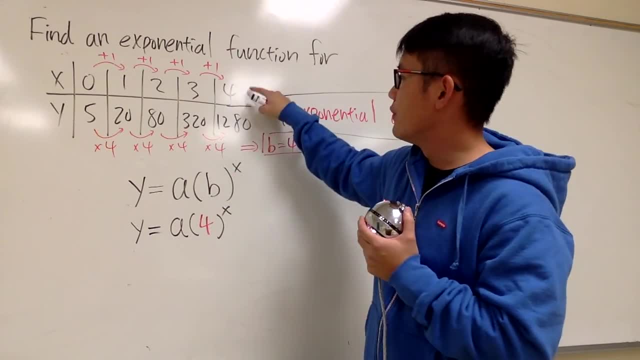 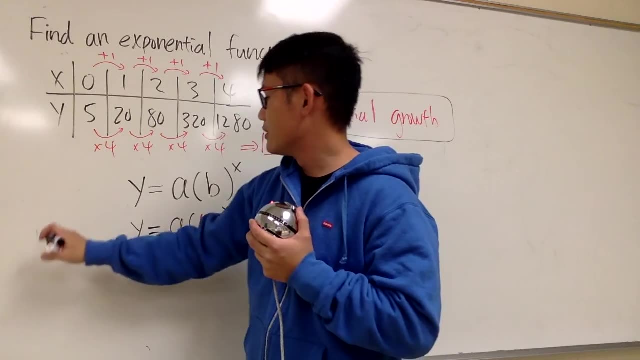 2 for x. y is 80.. Y can use 4 comma, 12, 80, up to you, But the easiest number to use will be this one: 0 and 5.. So I'm going to just say, I'm going to look at this and drag it. 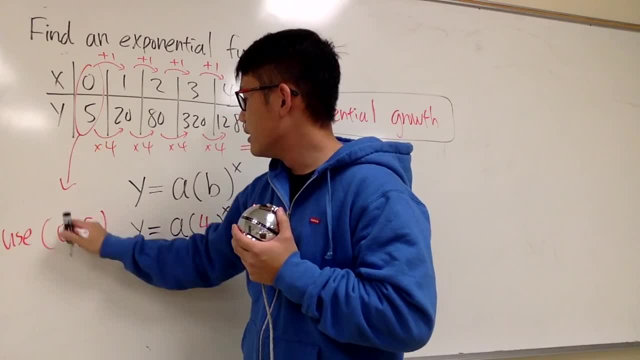 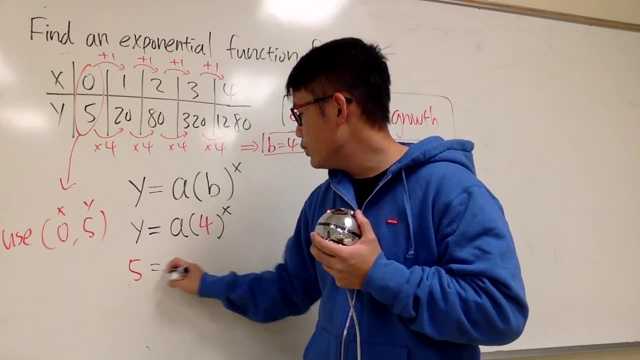 down. I will use 0 comma 5.. 0 for x, y is 5. And now I can just plug in 5 into y And this is equal to a- I don't know yet- times 4.. And the x is 80.. 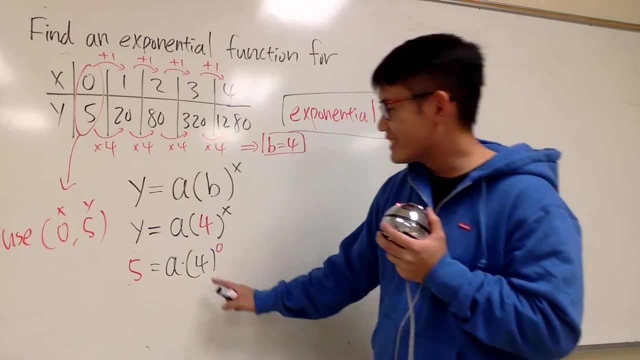 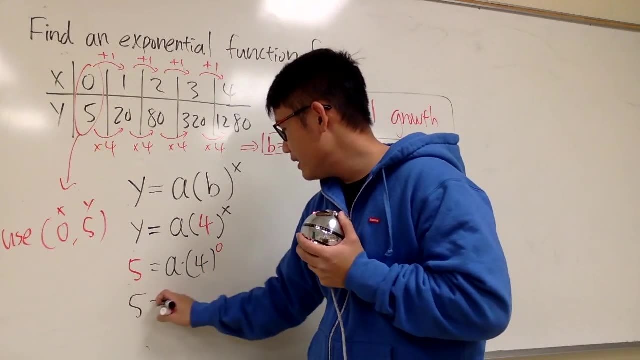 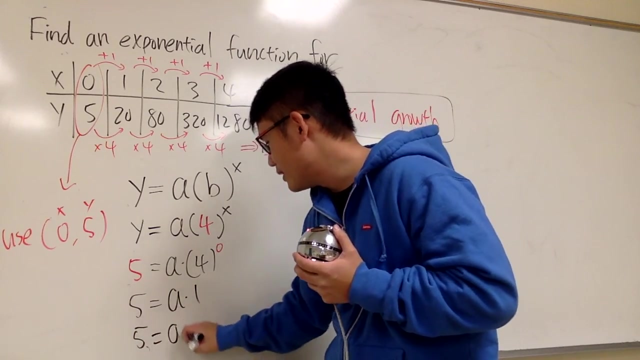 0. Why is this so easy? Because we have 4 to the 0's power is just a 1, right? So this is just 5, equals to a times 1.. a times 1 is just a. So this is just 5, is equal to a a. 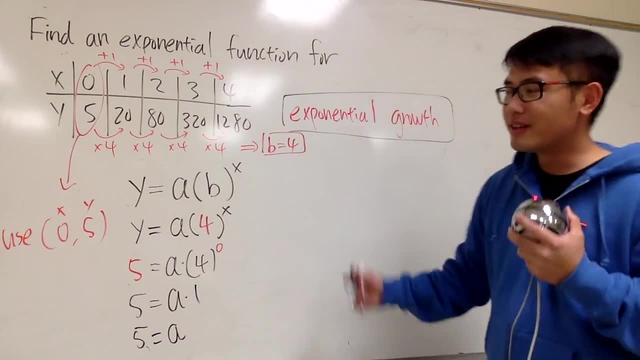 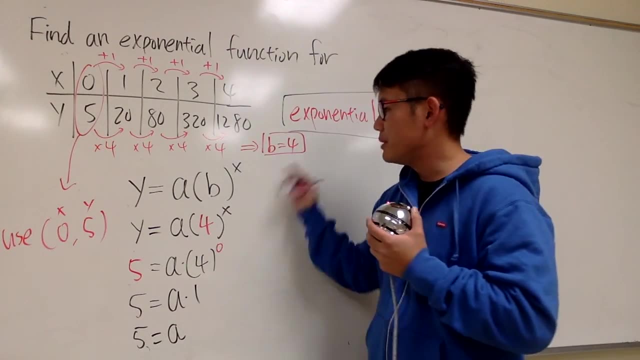 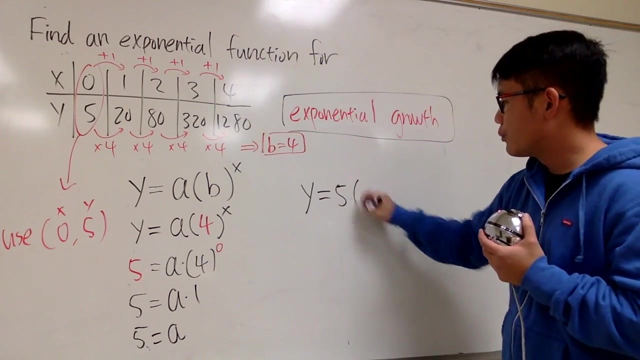 is equal to 5.. Same thing. Finally, the answer. Remember, whenever you're trying to write an equation or a function, the x and y stays And we plug in the a and b values in here And the answer it will be: y equals to a is 5, parentheses, b is 4.. And then the x is in. 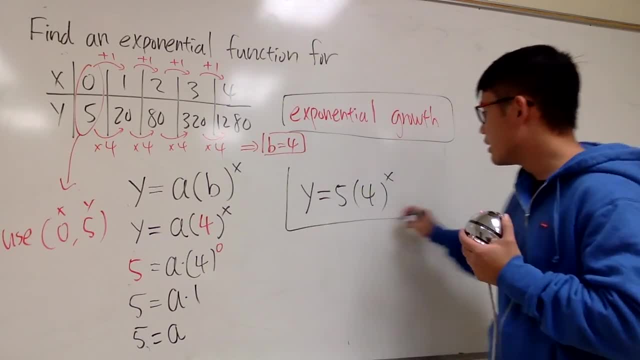 the exponent. That's why it's an exponential function. This is it.